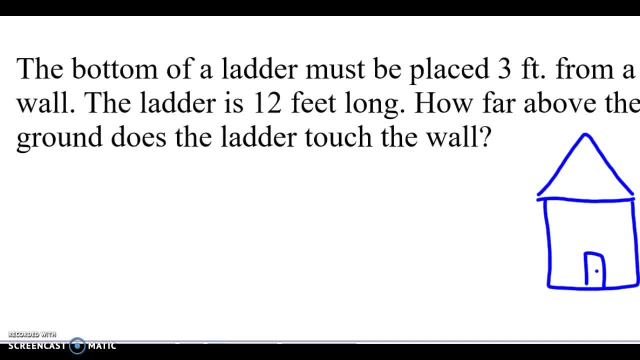 The bottom of the ladder must be placed three feet from the wall. So here is our wall. Alright, this is the wall. Okay, so your ladder must be placed three feet from the wall. The ladder itself is 12 feet long. Now, ladders typically lean up against a wall especially. 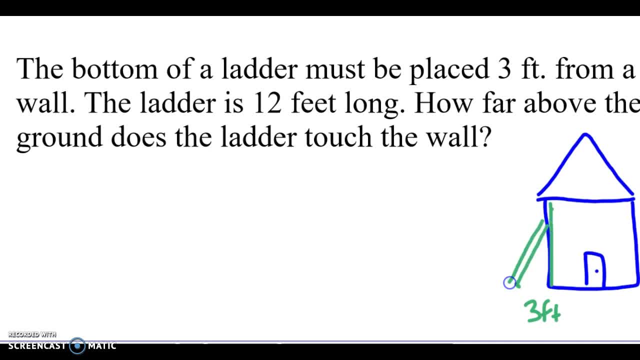 in these kinds of problems. So there's our ladder. Okay, you can make it an actual ladder if you want to, if it helps. So there's your ladder. It's got to touch the ground. So we know so far that it is three. 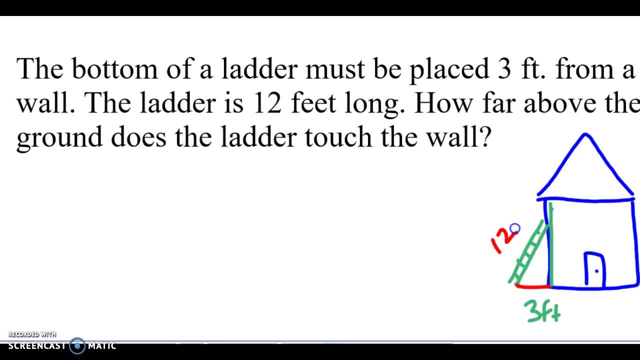 feet from the wall and the ladder is 12 feet long. Okay, how far above the ground does the ladder touch the wall? So how far above the ground is this touch point? So we know that this is our missing side. So now, just like before, you have to determine: are we trying to solve for A, B and C, All? 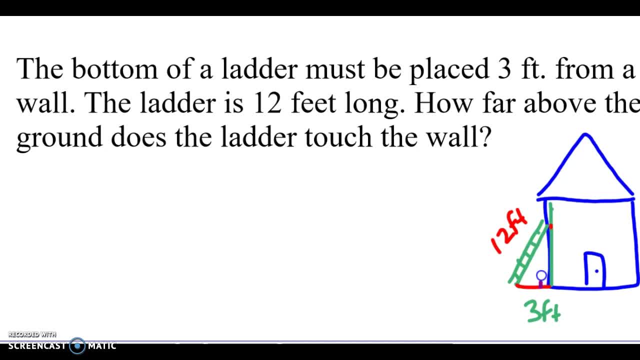 of these problems are going to give you a right triangle. So, as you can see, here's our 90 degree angle and that's going to point us to the letter C. Okay, so we know now that we have to solve for a leg. So Pythagorean theorem is: A squared plus B squared equals. 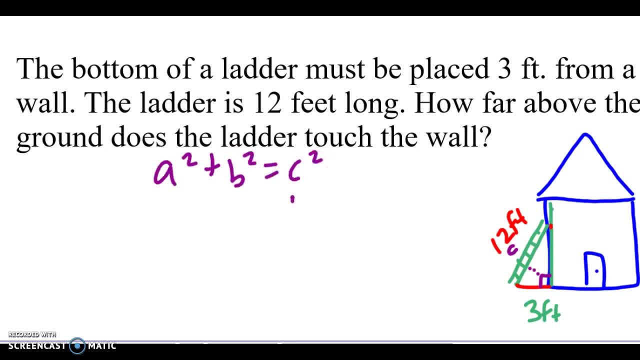 C squared, And C squared has to be your hypotenuse, So we're going to plug that in for C and then pick A or B for 3.. We'll just call it A, So we have 3 squared plus B squared equals 12 squared. Now you're. 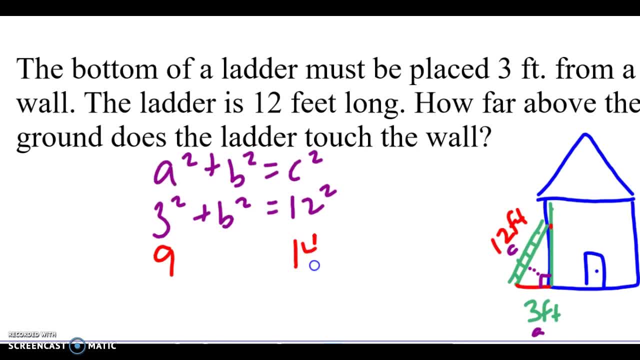 going to solve out your knowns. So that's going to be 9.. This will be 144.. And we still don't know. B. Oops, that's a plus sign. Oh goodness gracious. Okay, There we go All. 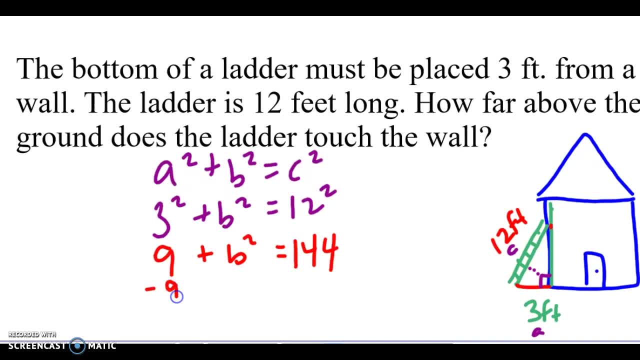 right now you're going to. you need to get B all by itself, So you're going to subtract the 9 from both sides of your equal sign: 144. take away 9 gives us 135, which is B squared. And then your final step is going to be to: 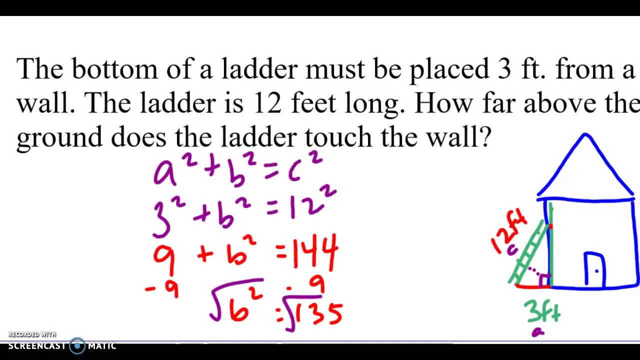 square root, square root. And again, you need the calculator for this one. Pardon me, I got to get mine started up again. Okay so the square root of 135 is 11.618, which we're going to round to 11.618.. 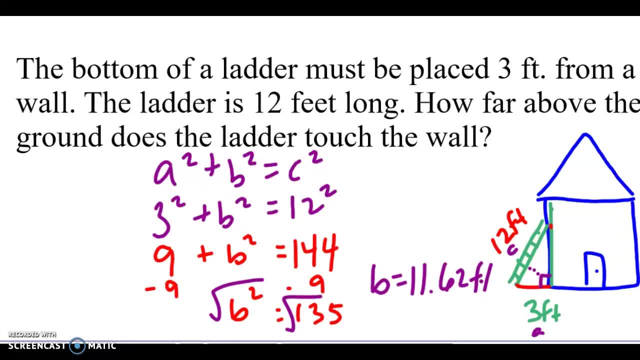 11.618.. 11.618., 11.618., 11.618. 11.618.. six, two feet. you have to put a unit of measure because this is a real world problem. it's not just eleven point six, two. it has to represent something in. 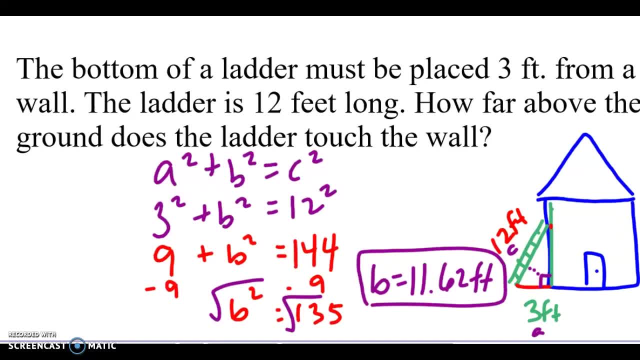 this case its feet. and then you just ask yourself if it makes sense this. so we're saying this wall, it reaches the wall at eleven point six, two feet, our ladders only twelve feet, so it's only a little bit taller if it were straight up and 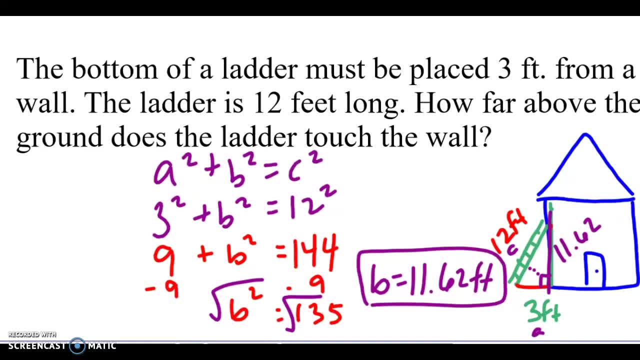 down against this wall right here. so what? it makes sense that a twelve foot ladder could be placed three feet against the wall and hit it. eleven, six, eleven point six feet. yeah, it's a little close but it works. okay. so that is our answer. so you just check it out. you can plug your numbers back in to see that. 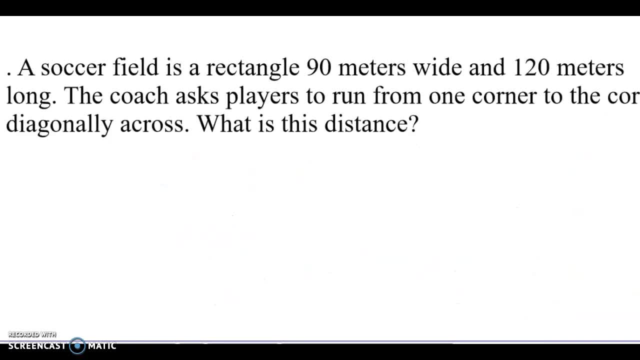 it's true, but if you calculated carefully you should be good to go all right. here's another example. a soccer field is a rectangle ninety meters wide and a hundred twenty meters long. the coach asks players to run from one corner to the corner diagonally across. what is the distance? so I know the. 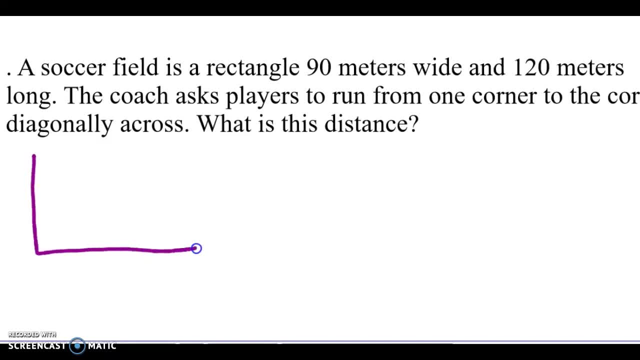 question is: what is the distance? so I know the question is: what is the distance? so I know the question is: what is the distance? so we've got many soccer players. so we've got many soccer players. so we've got many soccer players out there. here's a soccer field, okay, it? 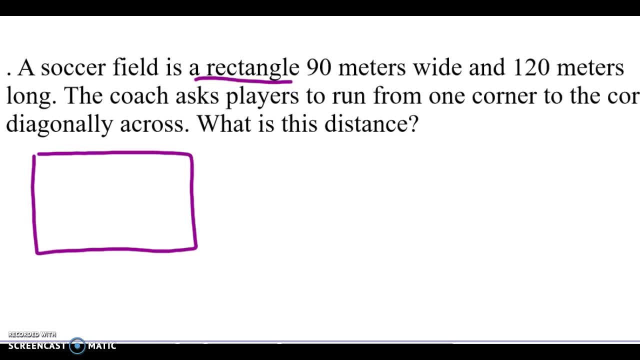 out there, here's a soccer field, okay. it out there, here's a soccer field, okay. it says: right here, it's rectangle, okay. 90 says right here, it's rectangle, okay. 90 says right here, it's rectangle, okay, 90 meters wide and 120 meters long. so 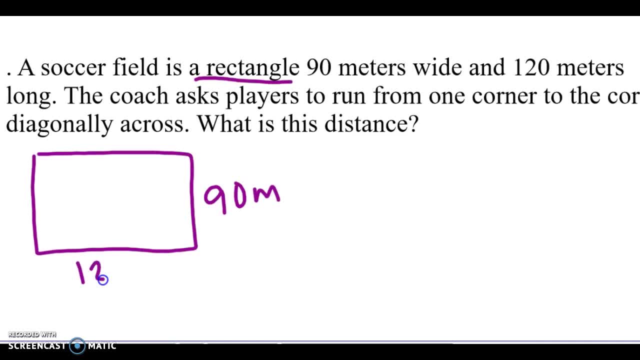 meters wide and 120 meters long. so meters wide and 120 meters long. so you've got our 90 meters here and our you've got our 90 meters here and our you've got our 90 meters here and our 120 meters here. now, that's not a triangle. 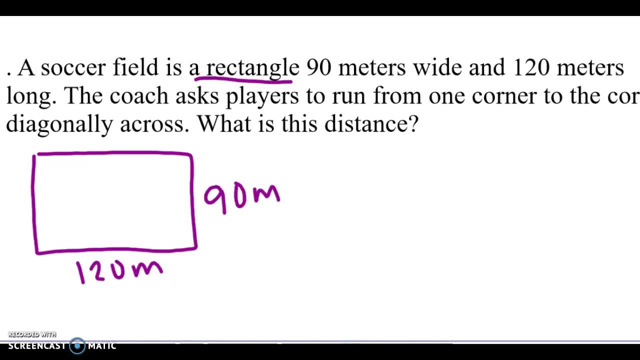 120 meters here, now, that's not a triangle. 120 meters here, now, that's not a triangle, okay. but if you think about the okay, but if you think about the okay, but if you think about the problem, you go back into it. the coach problem, you go back into it, the coach. 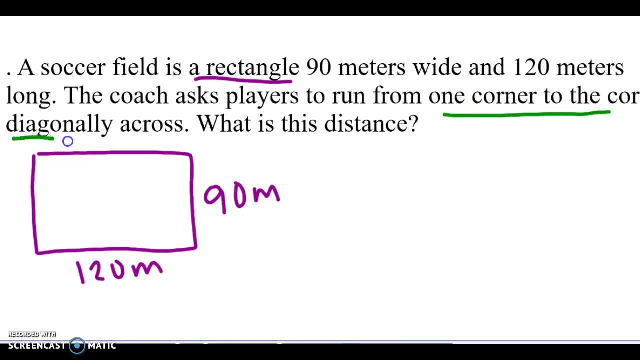 problem. you go back into it. the coach asks players to run from one corner to asks players to run from one corner to asks players to run from one corner to the corner diagonally across. so we've the corner diagonally across. so we've the corner diagonally across. so we've got our players here, okay, and they need. 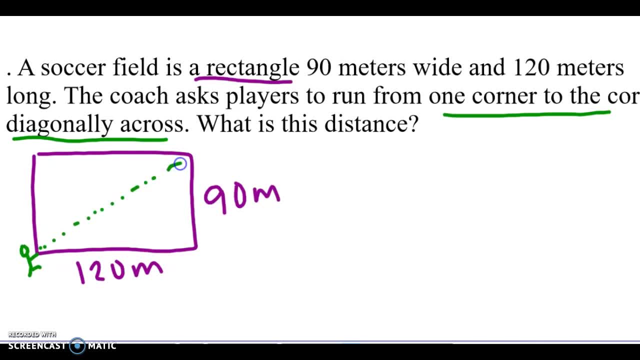 got our players here, okay, and they need got our players here, okay, and they need to run across the field here. we want to to run across the field here. we want to to run across the field here. we want to know how far they're running. so now we 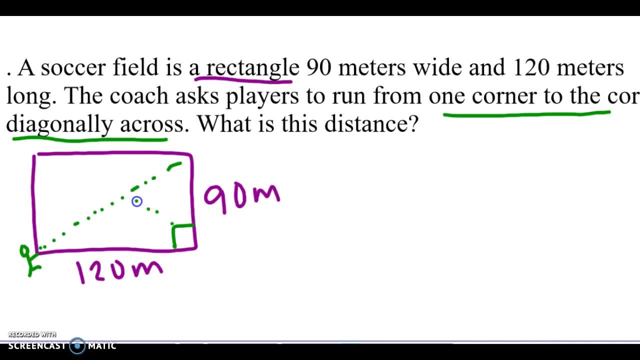 know how far they're running. so now we know how far they're running. so now we have our right triangle, we have our two, have our right triangle, we have our two, have our right triangle, we have our two measures and we are looking for the long measures and we are looking for the long. 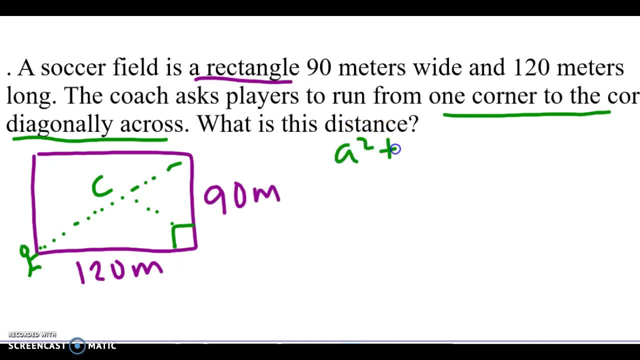 measures and we are looking for the long side. so you're gonna use a squared plus side. so you're gonna use a squared plus side. so you're gonna use a squared plus B squared equals C squared- now you're B squared equals C squared. now you're. 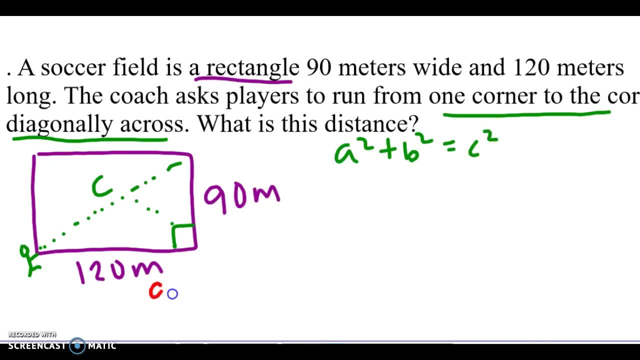 B squared equals C squared. now you're gonna take your numbers, plug them in. gonna take your numbers, plug them in. gonna take your numbers, plug them in. pick an a and a B again. it does not pick an a and a B again. it does not pick an a and a B again. it does not matter, just pick one. so we have 120. 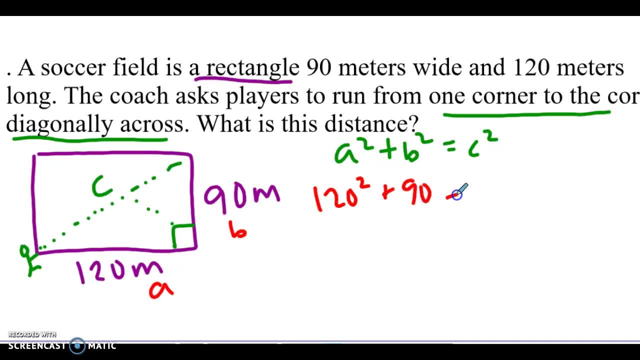 matter, just pick one. so we have 120. matter, just pick one. so we have 120 squared plus 90 squared whoops equals C squared. plus 90 squared whoops equals C squared. plus 90 squared whoops equals C squared. you're gonna have to solve these. 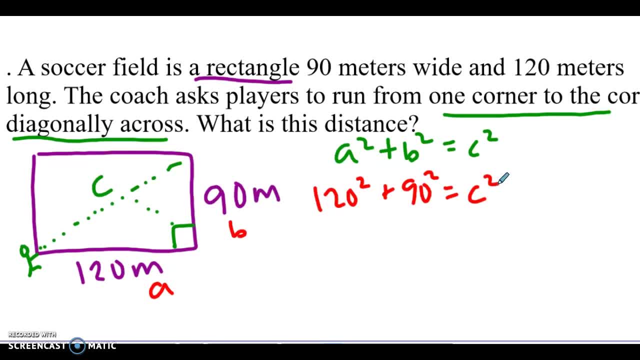 squared. you're gonna have to solve these squared. you're gonna have to solve these ones out. so we have 120 squared, which is ones out. so we have 120 squared, which is ones out. so we have 120 squared, which is fourteen thousand four hundred plus 90. 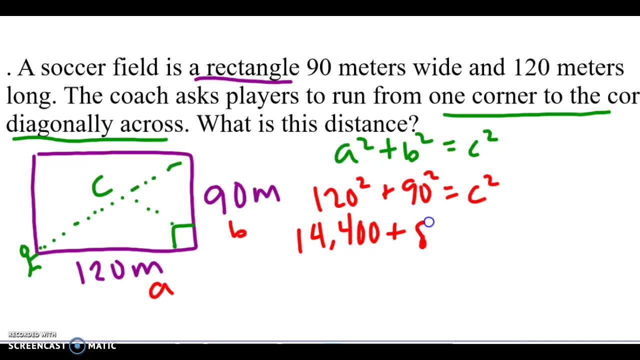 fourteen thousand four hundred plus 90, fourteen thousand four hundred plus 90 squared, which is eight thousand one squared, which is eight thousand one squared, which is eight thousand one hundred, equals C squared. you're gonna add hundred, equals C squared. you're gonna add hundred equals C squared. you're gonna add those two together, which is twenty. 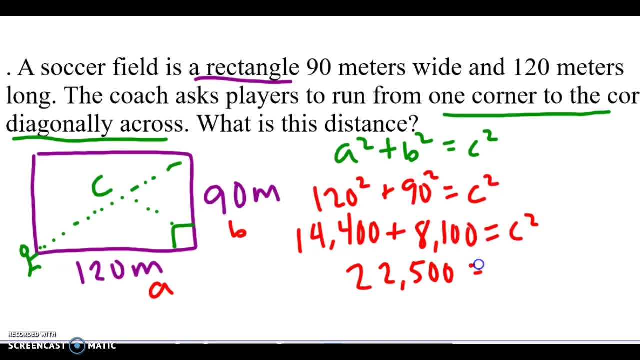 those two together, which is twenty. those two together, which is twenty two thousand five hundred, but that's still C two thousand five hundred, but that's still C two thousand five hundred, but that's still C squared. so your final step, as always. squared. so your final step, as always. 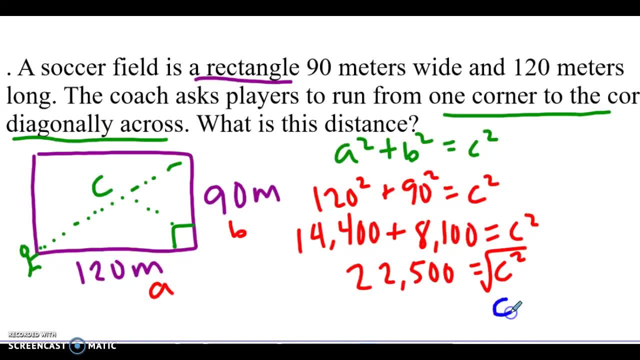 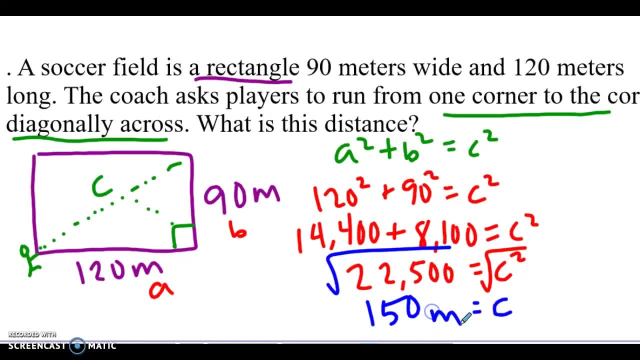 square root this, and that brings us to square root this, and that brings us to 150 meters. and again, just to check, make 150 meters. and again, just to check, make 150 meters. and again, just to check, make sure your numbers make sense. would it sure your numbers make sense, would it? 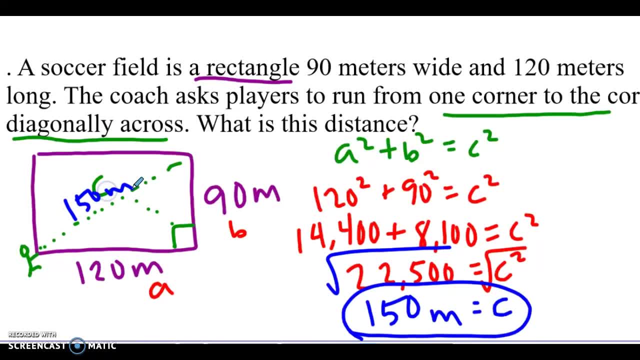 sure your numbers make sense. would it make sense that they would have to run? make sense that they would have to run? make sense that they would have to run about a hundred and fifty meters, if the about a hundred and fifty meters, if the about a hundred and fifty meters, if the field was this size? I think so all. 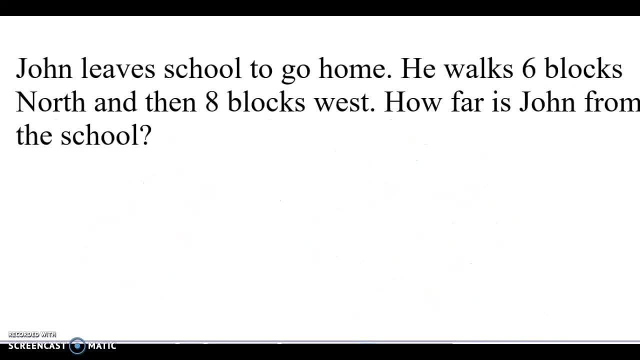 field was this size? I think so. all field was this size? I think so, all right. one final example. John leaves right. one final example: John leaves right. one final example: John leaves school to go home. he walks six school to go home. he walks six school to go home. he walks six blocks north and eight blocks west. how? 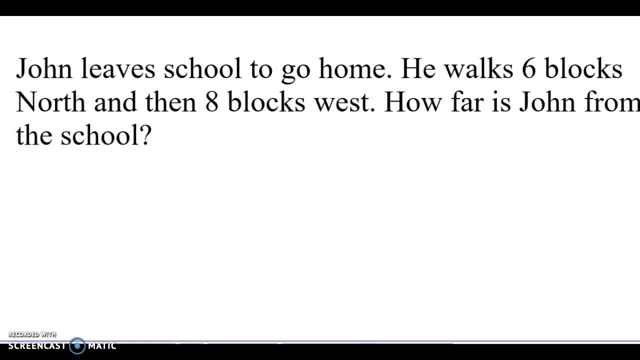 blocks north and eight blocks west. how blocks north and eight blocks west. how far is John from the school? so to know. far is John from the school? so to know. far is John from the school, so to know our coordinates. we have north, south and our coordinates. we have north, south and 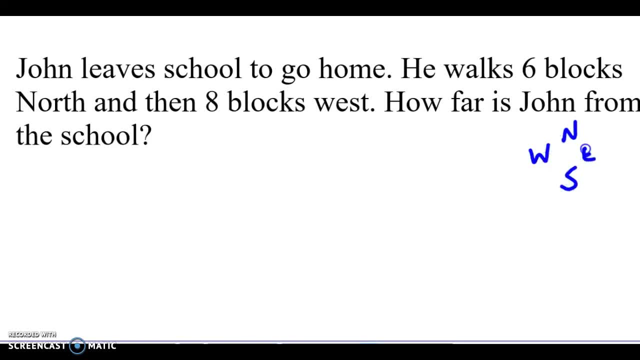 our coordinates. we have north, south and then east and west. I always learned it, then east and west. I always learned it, then east and west. I always learned it spells out the word we okay. so there's spells out the word we okay. so there's spells out the word we okay. so there's a little helpful hit. so he's gonna walk. 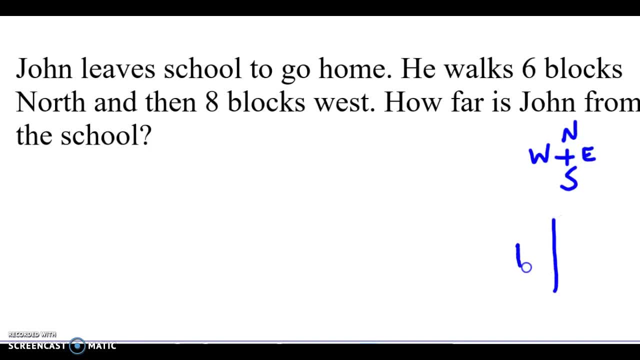 a little helpful hit, so he's gonna walk. a little helpful hit, so he's gonna walk six blocks north and then eight blocks. six blocks north and then eight blocks, six blocks north and then eight blocks west. whoops, I do that backwards west. whoops, I do that backwards. 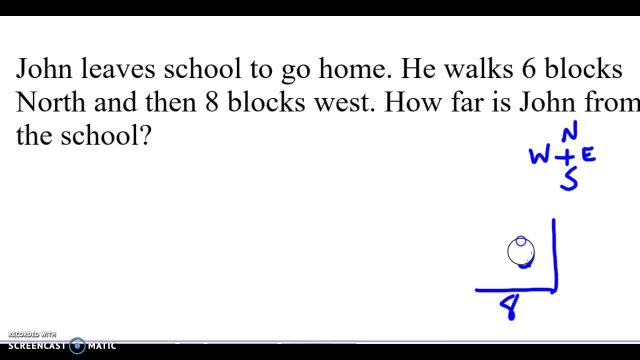 west. whoops, I do that backwards. so let me actually rewrite this six over. so let me actually rewrite this six over. so let me actually rewrite this six over here. how far is he from the school, so he here. how far is he from the school, so he? 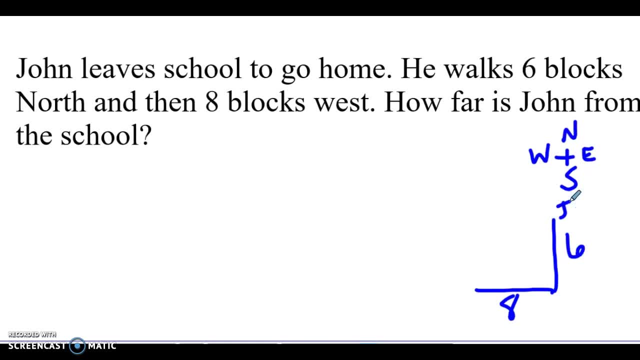 here. how far is he from the school? so he started here. this is where John is okay. started here. this is where John is okay. started here. this is where John is okay and he's leaving school, so we'll do. and he's leaving school, so we'll do. 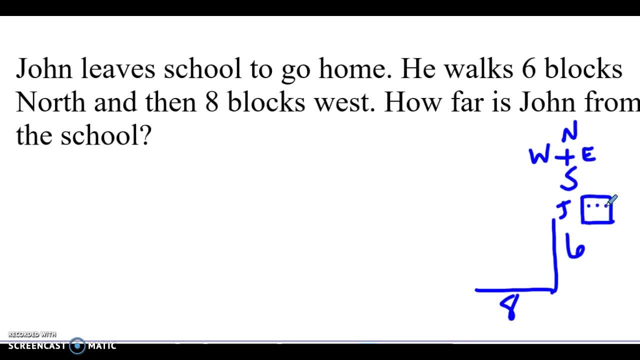 and he's leaving school. so we'll do schools a rectangle a little. those are I. schools a rectangle a little, those are I. schools a rectangle a little. those are- I don't know what those are- windows, don't know what those are. windows. don't know what those are windows. there's a school, here's his home. so 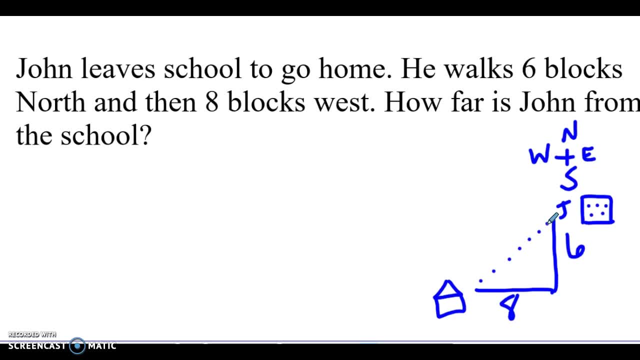 there's a school here's his home. so there's a school here's his home. so that's what he walked. we want to see how that's what he walked. we want to see how that's what he walked. we want to see how far he actually is from the school. so 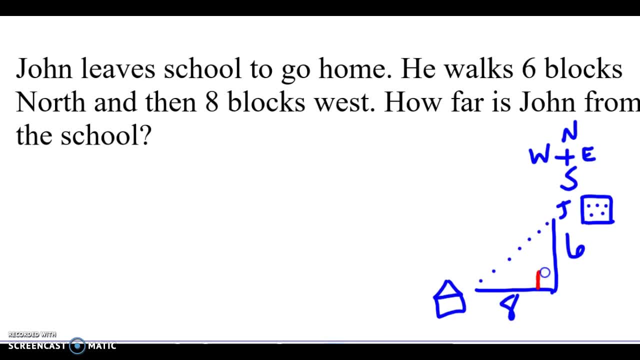 far he actually is from the school, so far he actually is from the school. so we have to establish our right triangle. we have to establish our right triangle. we have to establish our right triangle, our right angle in the triangle, so we, our right angle in the triangle, so we. 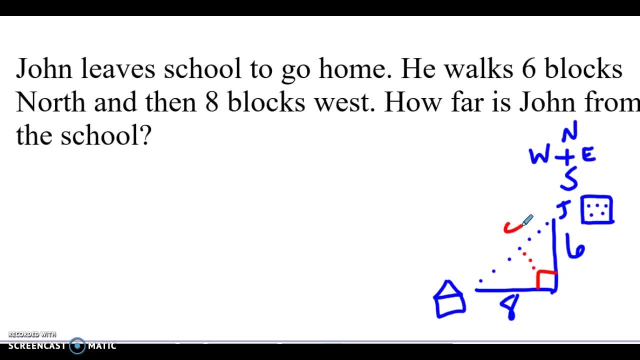 our right angle in the triangle. so we are looking for C. okay, so you're gonna are looking for C. okay, so you're gonna are looking for C. okay, so you're gonna. use a squared plus B squared equals C. use a squared plus B: squared equals C. 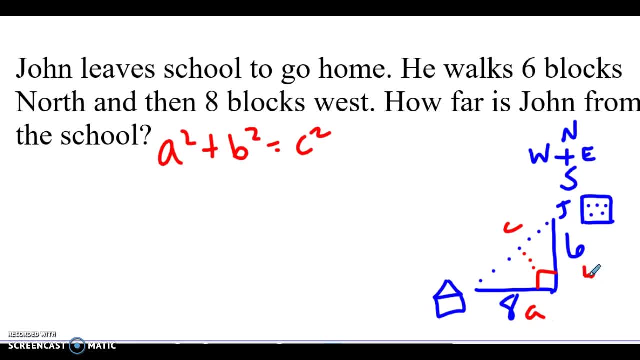 use: a squared plus B squared equals C squared. pick an a. pick a B- 8 squared squared. pick an a. pick a B- 8 squared squared. pick an a. pick a B. 8 squared plus 6 squared equals C squared 64 plus plus 6 squared equals C squared 64 plus. 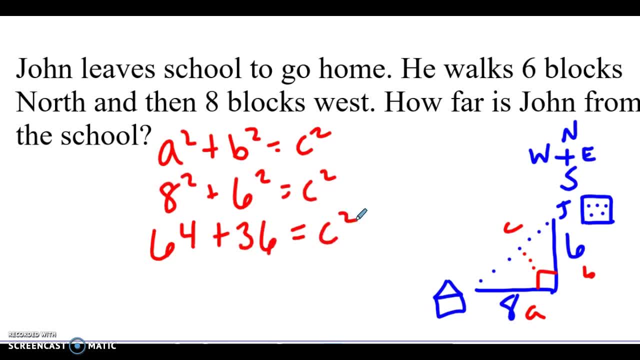 plus 6 squared equals C squared. 64 plus 36 equals C squared, and this is going to 36 equals C squared. and this is going to 36 equals C squared. and this is going to calculate to 100, which, if you've been calculate to 100, which, if you've been,